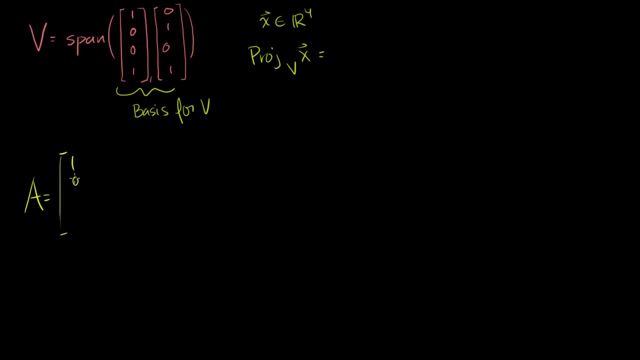 subspace. so let's say A is equal to 1, 0, 0, 1, 0, 1, 0, 1, so A is a matrix whose columns are the basis for a subspace. then the projection of x. 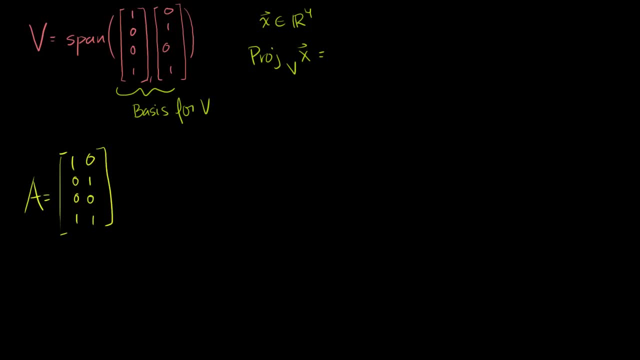 onto V would be equal to: and this is kind of hard. the first time you look at it it gives you a headache, but there's a certain pattern or symmetry or a way of you could say: it's A times you're going to have something in the middle and 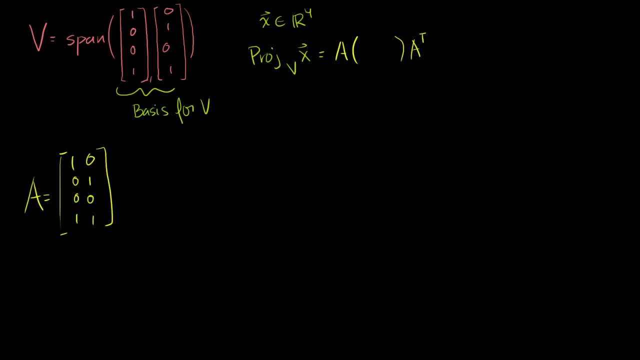 then you have A transpose times your vector x And the way I remember it is in the middle you have these two guys switched around. so then you have A transpose A and you take the inverse of it. So you probably won't be using this in your everyday life. five: 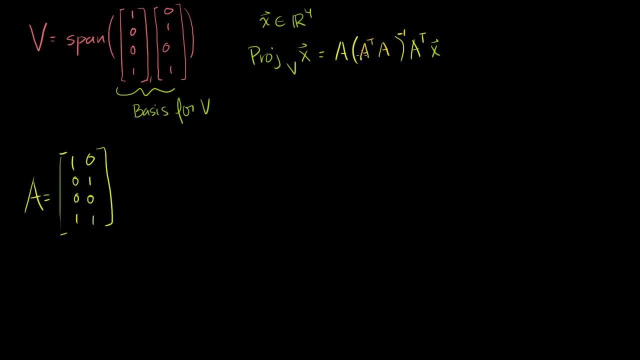 or ten years from now. so it's OK if you don't memorize it, but temporarily put this in your medium-term memory, because it's a good thing to know for doing these projection problems. So if we want to find the general matrix for this, 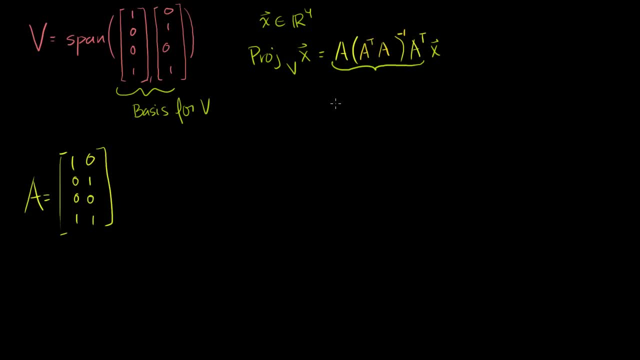 transformation. we just have to determine what this matrix is equal to, And that's just a bunch of matrix operations. So that's A. What is A transpose? A transpose is going to be A transpose. A transpose is going to be equal to just all the rows. 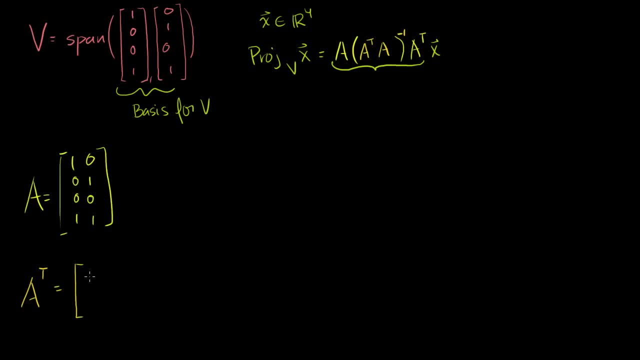 turned to columns. So the first column becomes the first row, So it becomes 1, 0, 0, 1.. Second column becomes the second row 0, 1, 0, 1.. That's what A transpose is. 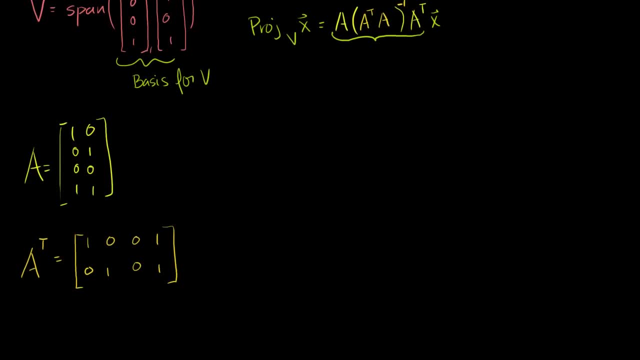 Now, what's A transpose A? To figure out that, I want to figure out what A transpose times A is, So let me multiply A transpose times A, So I'll rewrite A right here: 1, 0, 0, 1, 0, 1, 0, 1.. 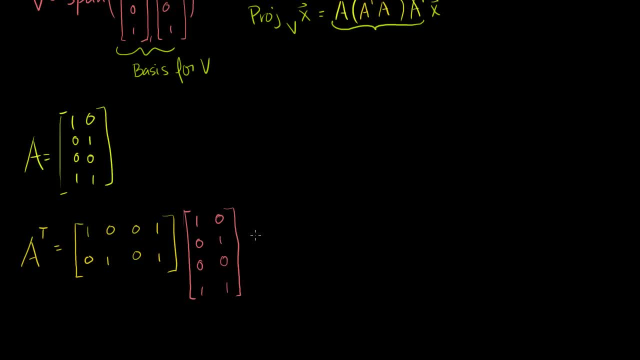 This will give us some good practice on matrix-matrix products. This is going to be equal to what? Well, first of all, this is a 2 by 4 matrix and I'm multiplying it by a 4 by 2 matrix. 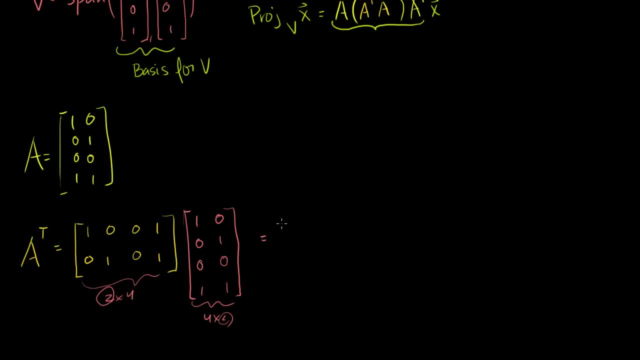 So it's going to be a 2 by 2 matrix. So the first entry is essentially the dot product of that row with that column. So it's 1 times 1 plus 0 times 0 plus 0 times 0 plus 1 times 1.. 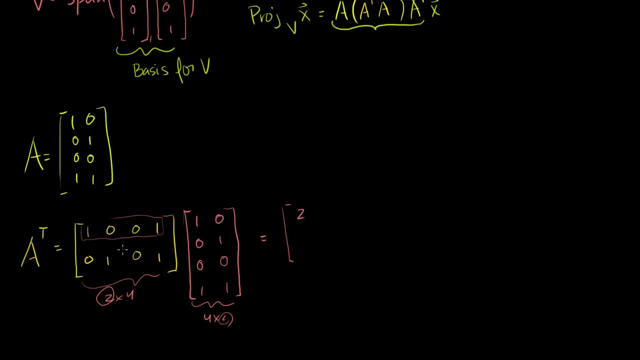 So it's just going to be 2 for that first entry right there, And then you take the dot product of this guy with this guy right here. So it's 1 times 0, which is 0,, plus 0 times 1,, which is 0,. 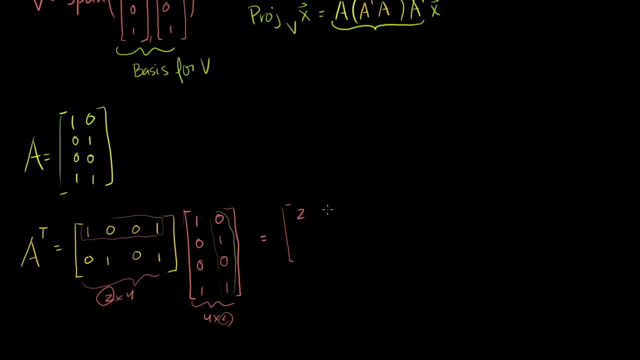 plus 0 times 0,, which is 0,, plus 1 times 1,, which is 1.. Now we do this guy, This guy dotted with this column right there: 0 times 1 is 0, plus 1 times 0 is 0,. plus 0 times 0 is 0, plus. 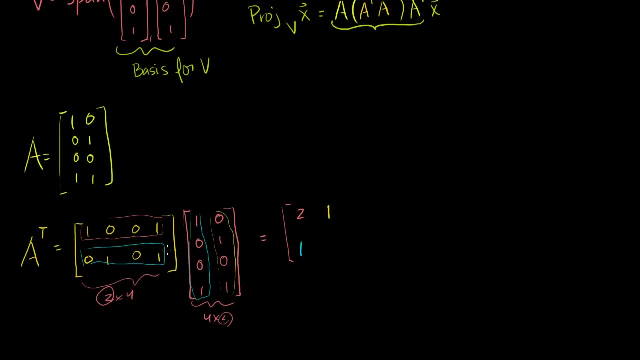 1 times 1 is 1.. And then, finally, this row dotted with this second column. second row with second column: 0 times 0 is 0,. 1 times 1 is 1,. 0 times 0 is 0,. 1 times 1 is 1.. 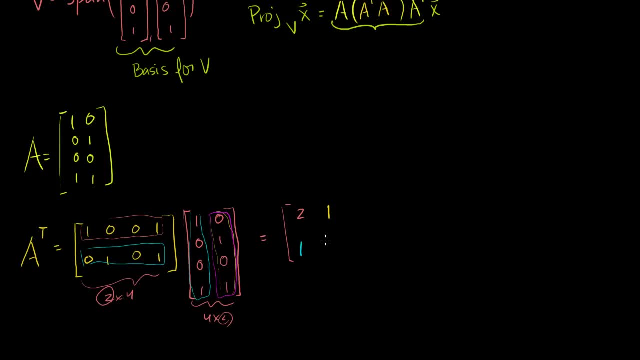 So we have: 1 times 1 is 1.. 1 plus 1 times 1.. So it's going to be 2.. It's going to be equal to 2.. So this right here, that right, there is A transpose A. 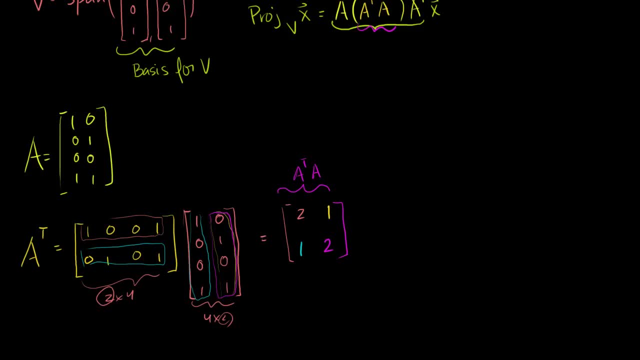 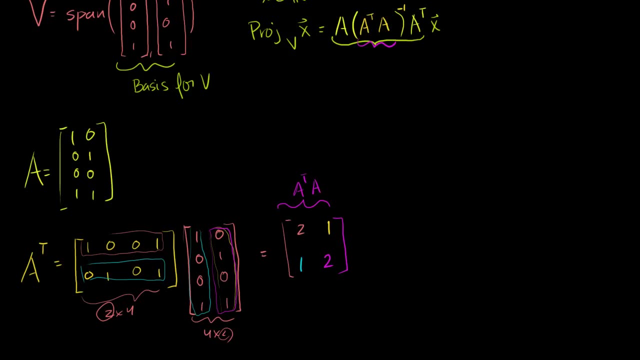 But that's not good enough. We need to figure out what the inverse of A transpose A is. This is A transpose A, but we need to figure out A transpose A inverse. So what's the inverse of this? So let me write it here. 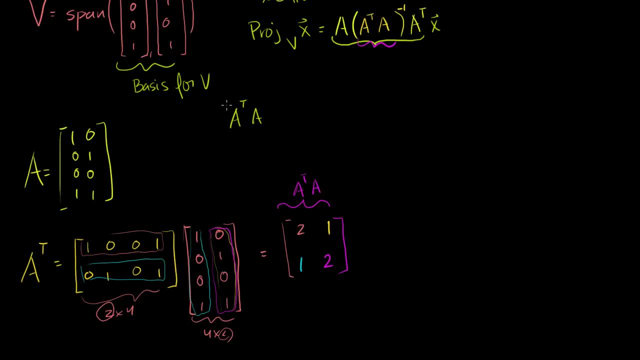 The inverse. A transpose, A inverse is going to be equal to what It's 1 over the determinant of this guy. And what's the determinant here? It's going to be 1 over the determinant of this. The determinant is 2 times 2, which is 4, minus 1 times 1.. 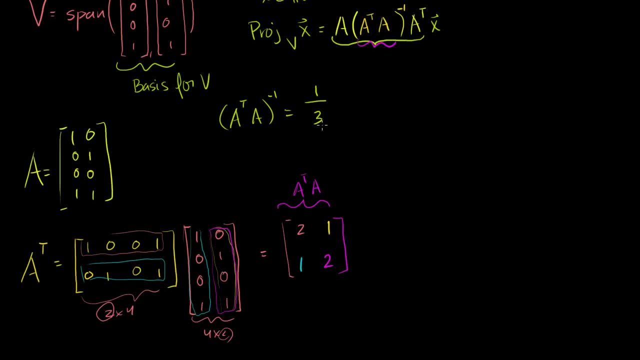 So it's 4 minus 1, which is 3.. So 1 over the determinant times. this guy where if I swap these two, so I swap the 2's, So this 2 goes here And then this orange 2 goes over here. 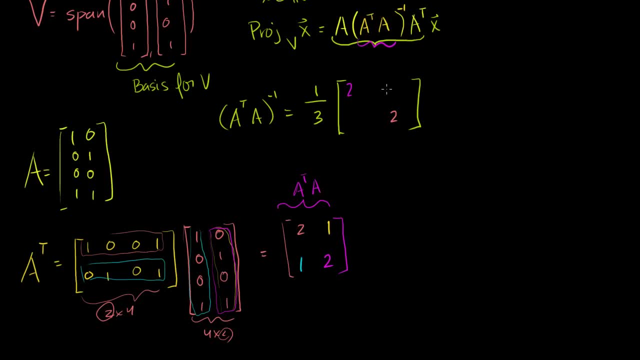 And then I make these 1's negative, So this becomes a minus 1, and this becomes a minus 1.. We learned that this is a general solution for the inverse of a 2 by 2 matrix. I think it was 10 or 11 videos ago. 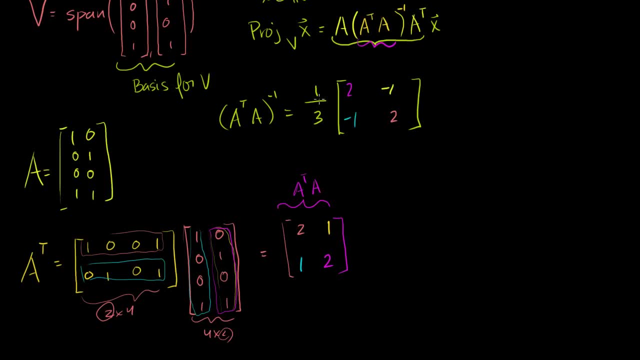 And you probably learned this in your Algebra 2 class, frankly. But there you go. We have A transpose, A inverse, So we have this guy, We have this whole guy here. It's just this matrix. I could multiply, I could multiply the 1 third into it, but I don't have to do. 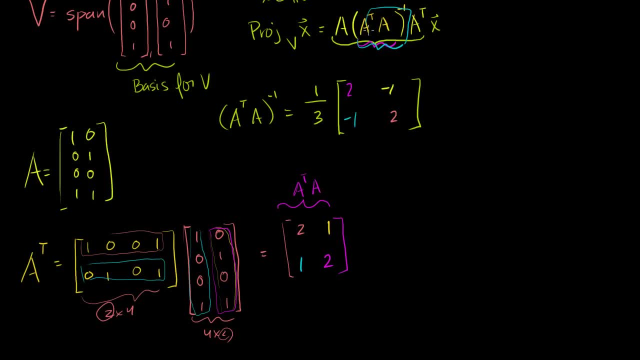 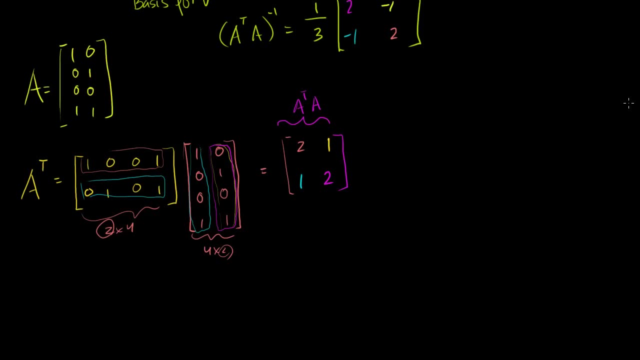 that just yet. But let's figure out the whole matrix now, The whole A times this guy: A transpose, A inverse times A transpose. So let me write it this way: So the projection onto the subspace V of x is going to be: 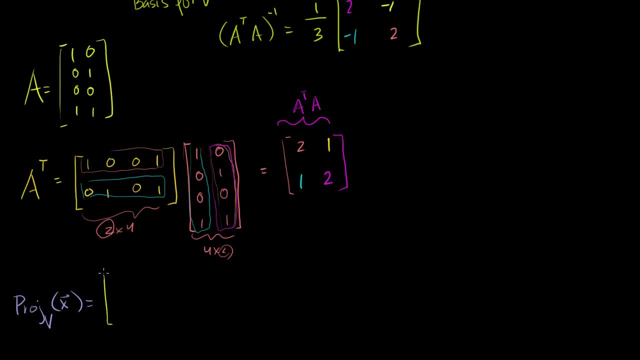 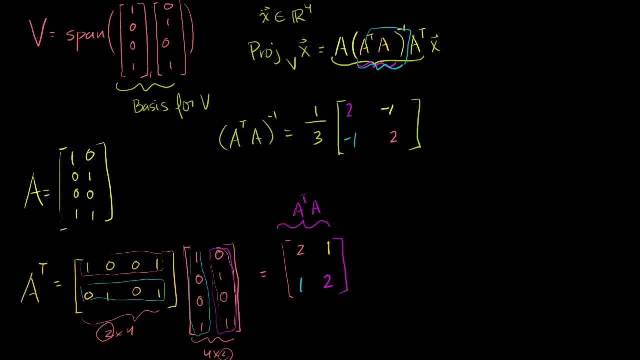 equal to A. Let me write it a little bit bigger like this: So 1001 0101 times A transpose A inverse. right A times A transpose A inverse. Which is this guy right here, And let's just put the 1 third out front, just because that's. 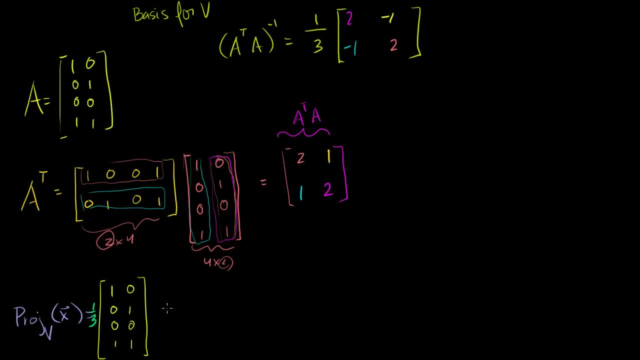 just a scalar, So I'll put the 1 third out front times this guy, This A transpose: A inverse is 1 third of A Inverse is 1 third times 2, minus 1, minus 1, 2.. 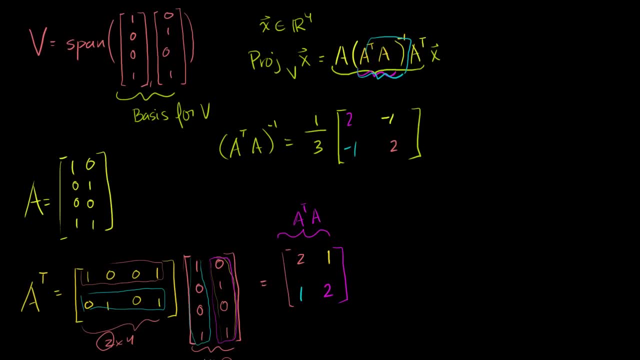 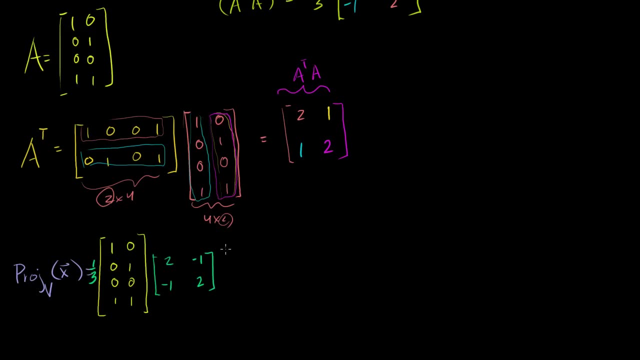 And then I'm going to multiply. it times A transpose, and all of that times our vector x. So A transpose is right there. It is 1, 0, 0, 1, 0, 1, 0, 1.. 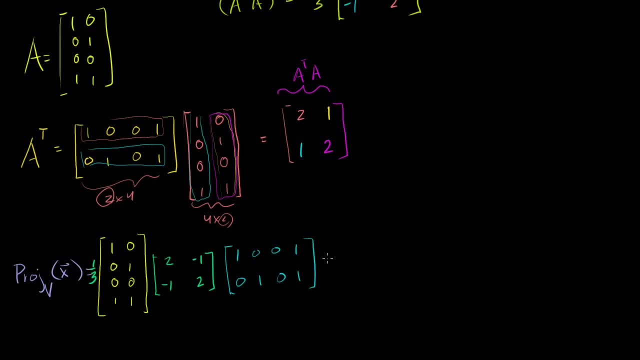 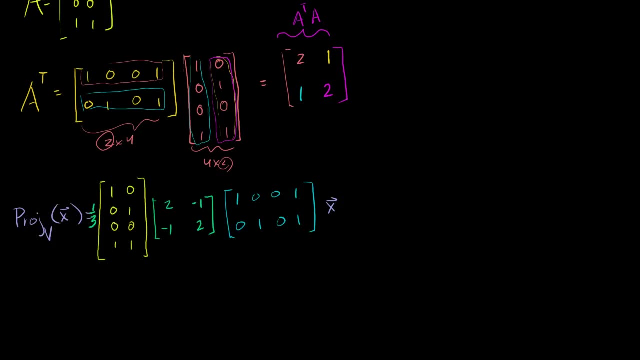 And then all of that's going to be times your vector x. So we still have some nice matrix, matrix products ahead of us. Let's see if we can do these. So the first one: let's just multiply these two guys. Let's multiply those two guys. 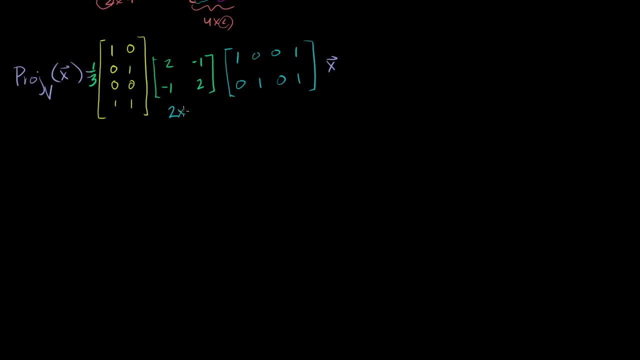 I don't think there's any simple way to do it. So this is a 2 by 2 matrix and this is a 2 by 4 matrix. So when I multiply them, I'm going to end up with a 2 by 4. 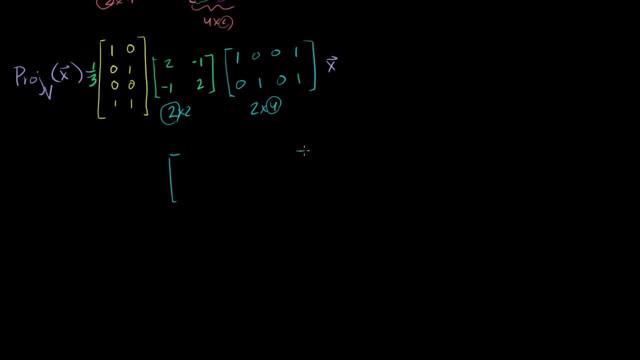 matrix. So let me write that 2 by 4 matrix right here, And then I can write this guy right here: 1, 0, 0, 1, 0, 1, 0, 1.. And then I have the 1 third that was from A transpose A. 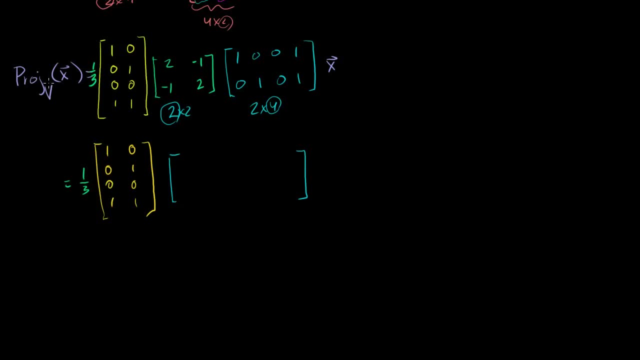 inverse, but I put the scaling factor out there And all of this is equal to the projection of x onto v. So let's do this product. So this first entry is going to be 2 times 1, plus minus 1 times 0.. 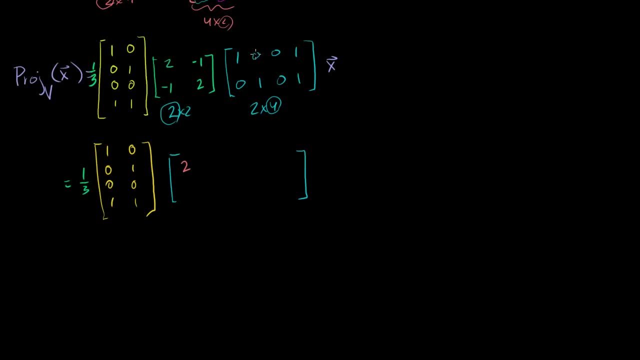 So that is just 2.. Then you're going to have 2 times 0, plus minus 1 times 1.. Well, that's minus 1.. Then you're going to have 2 times 0, plus minus 1 times 0.. 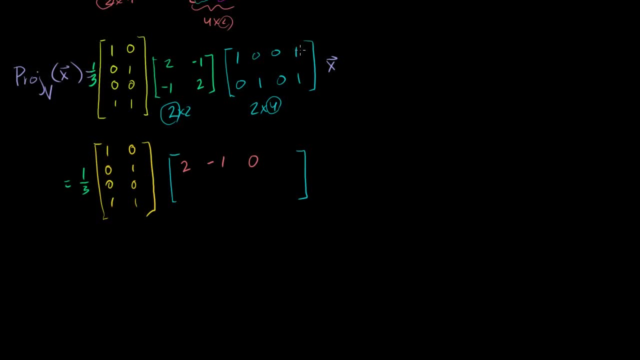 Well, that's just 0.. And then you're going to have 2 times 1, plus minus 1 times 1.. That's 2 minus 1.. That's just 1, right, 2 times 1, plus minus 1 times 1.. 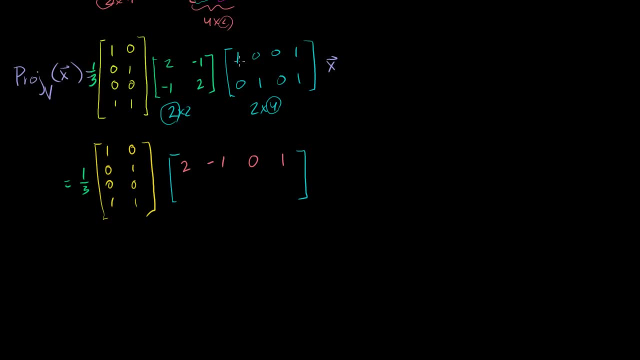 Fair enough, Now let's do the second row: Minus 1 times 1, plus 2 times 0.. So that's just minus 1.. Minus 1 times 1.. times 0 plus 2 times 1.. 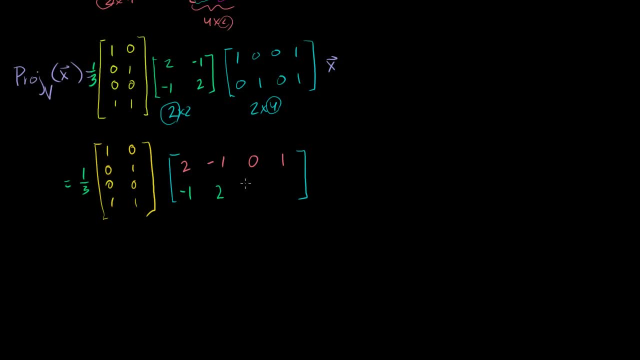 Well, that's just 2.. Minus 1 times 0 plus 2 times 0, that's just 0.. Minus 1 times 1 plus 2 times 1.. Well, that's minus 1 plus 2.. 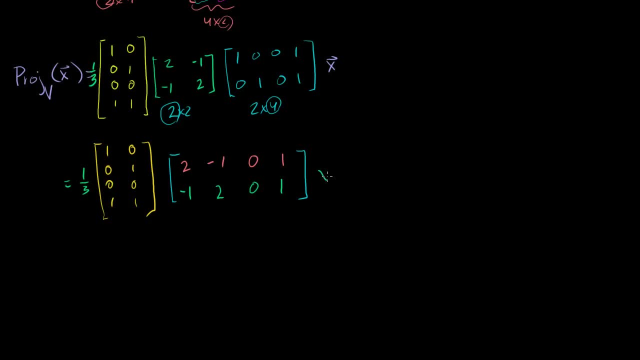 So that is 1. Almost there. And of course we have to multiply times x at the end. That's what the transformation is. But this right here is our transformation matrix. One more left to do. Let's hope I haven't made any careless mistakes and that I 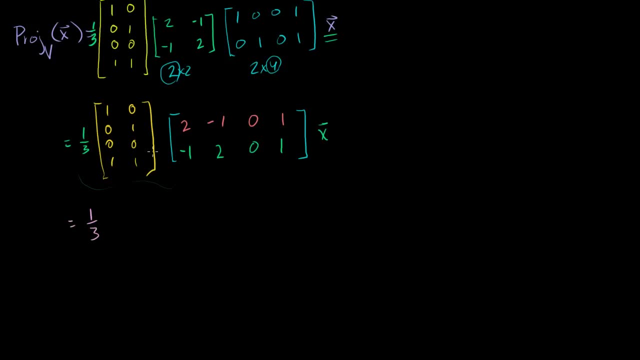 won't make any when I'm doing this product, Because this is going to be a little more complicated, Because this is a 4 by 2 times a 2 by 4, I'm going to end up with a 4 by 4 matrix. 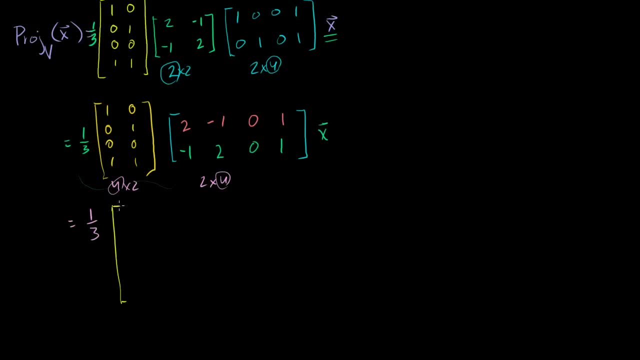 So let me give myself some breathing room here, because I'm going to generate a 4 by 4 matrix right there, And so what am I going to get? So this first entry is going to be 1 times 2 plus 0 times. 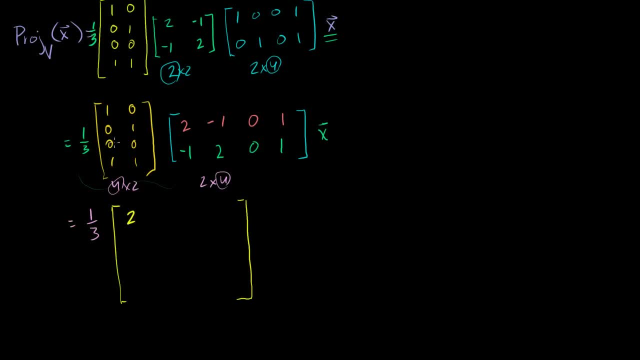 minus 1.. So it's just going to be 1 times 2 plus 0 times minus 1.. It's going to be equal to 2.. The next entry this row times any column. here is just going to be the first entry in the column right. 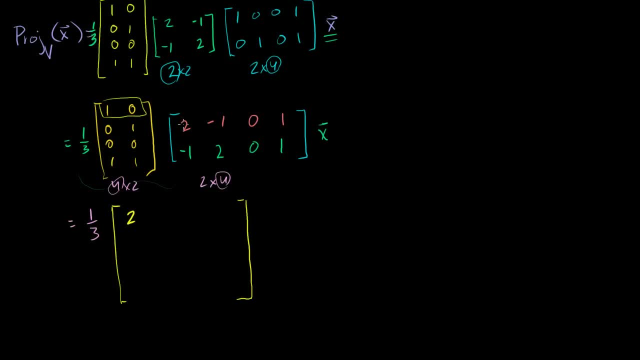 Because it gets zeroed out. So 1 times 2 plus 0 times minus 1 is just 2.. 1 times minus 1 plus 0 times 2 is just minus 1.. 1 times 0 plus 0 times 0 is 0.. 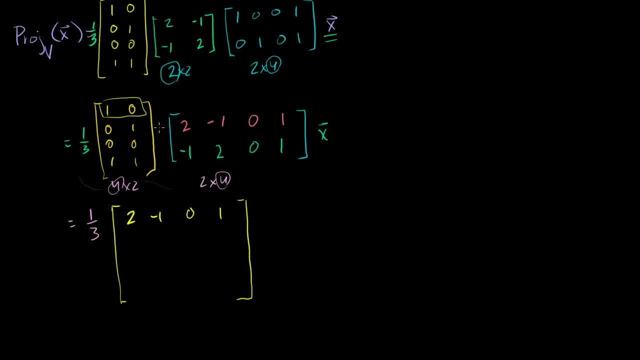 1 times 1 plus 0 times 1 is just 1.. When you take this row and you multiply, it times these columns. you literally just got your first row There. Now let's do this: row times these columns. Now you've got a 0 here, so you're going to have a 0 times. 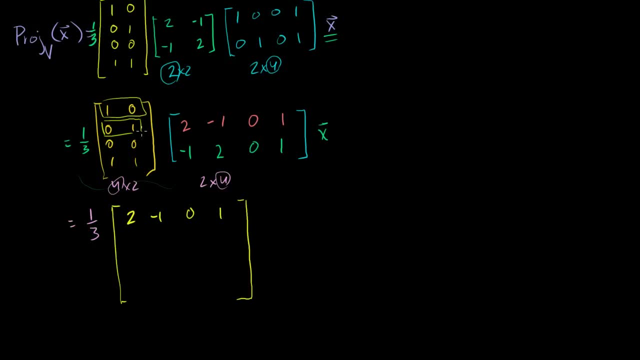 the first entry of all of these and a 1 times the second one. So 0 times 2 plus 1 times minus 1 is minus 1.. 0 times minus 1 plus 1 times 2 is 2.. You're just going to get the second row here. 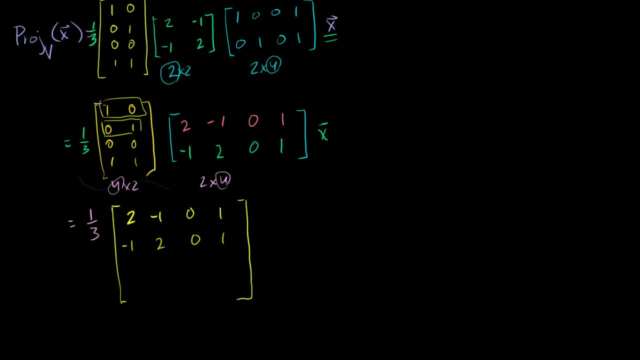 2, 0, 1.. And that actually makes sense because if you just look at this part of the matrix, it's the 2 by 2 identity matrix. So anyway, That's a little bit more complicated, OK. 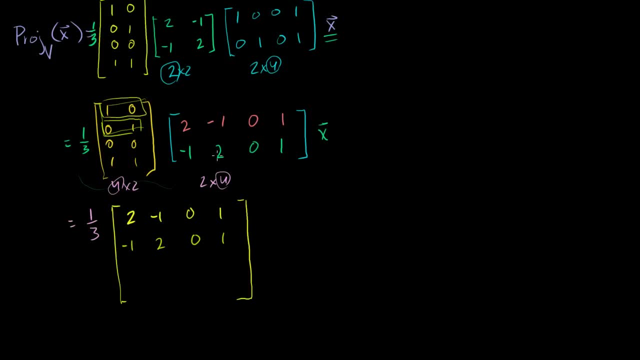 OK. OK, That's a little hint why this looks very much like that, But we're just going to go through this matrix product. Now you multiply this. Let me do it in a different color. You multiply this guy times each of these columns. 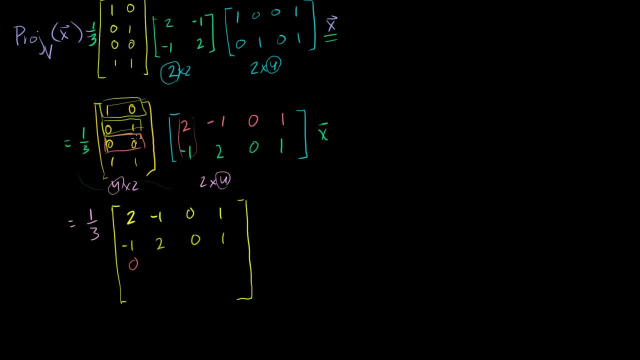 That guy dotted with that is just going to be 0, because this guy is essentially the 0 row vector. So you're just going to get a bunch of 0's And then finally this last row. it's 1 times the first. 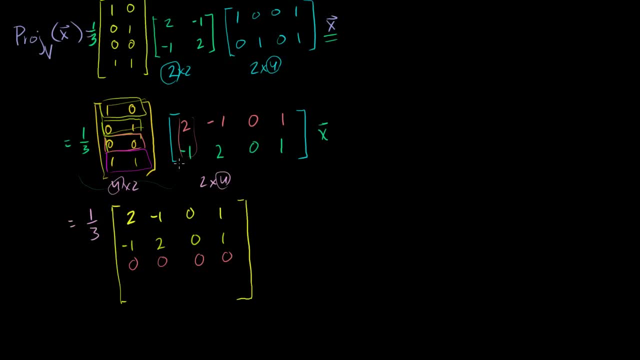 entry plus 1 times the second entry. So this guy's going to be 2 plus minus 1, which is 1., Minus 1 plus 2, which is 1.. 0 plus 0, which is 0.. 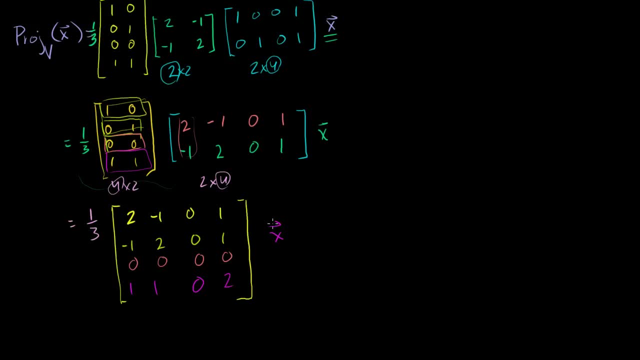 And then 1 plus 1, which is 2.. And all of that times x. And there you have it. This is exciting. The projection onto v of x is equal to this whole matrix times x. So this thing, right here I could multiply the 1 third. 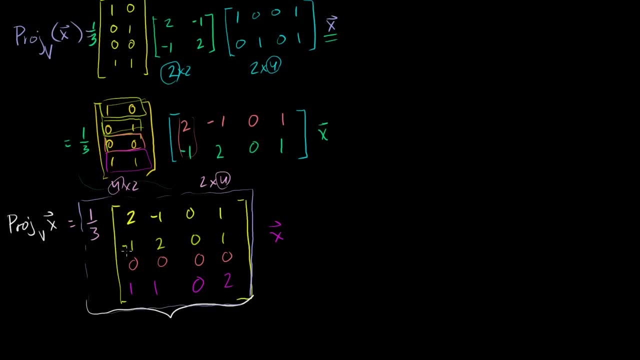 into it, but we don't have to do that. That'll just make it a little bit more messy. This thing right here is the transformation matrix And, as you can see, since we're transforming, remember this projection onto v- this is a linear transformation. 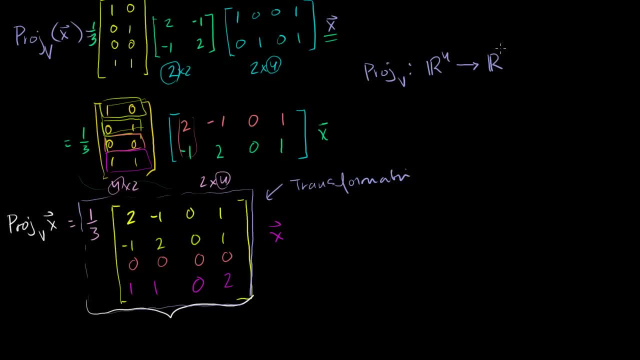 from R4 to R4.. You give me some member of R4, and I'll give you another member of R4 that's in my subspace. That is the projection. So this is going to be a 4 by 4 matrix.